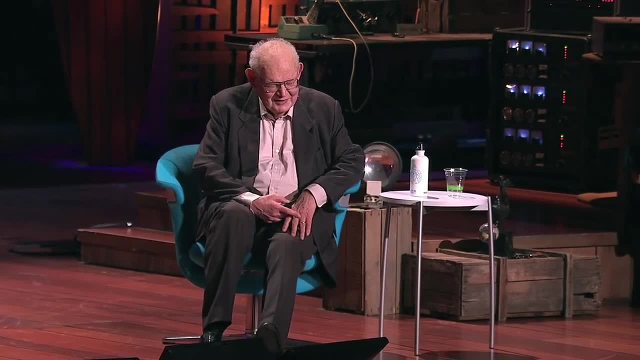 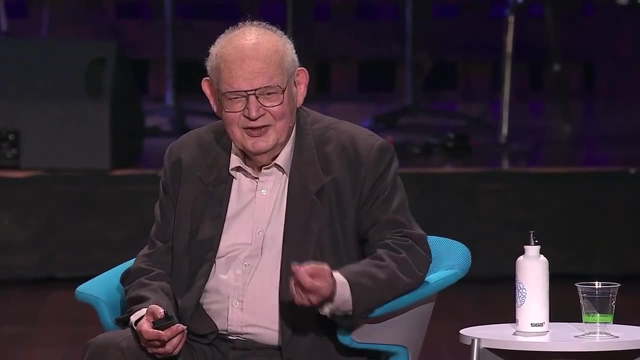 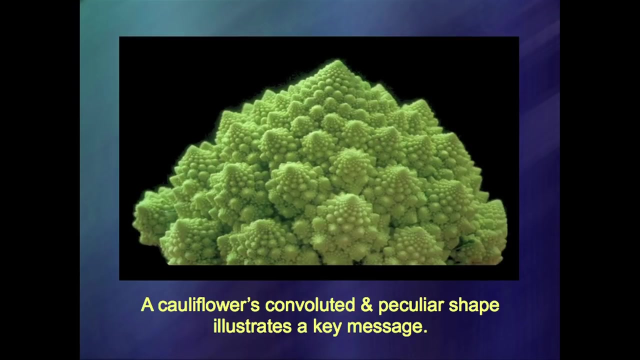 to somebody who has had Latin in my long past, use means the country of regularity, But it is not so. Regularity is a country of roughness, because the basic aspect of the world is very rough. So let me show you a few objects, some of them artificial, other of them very real. 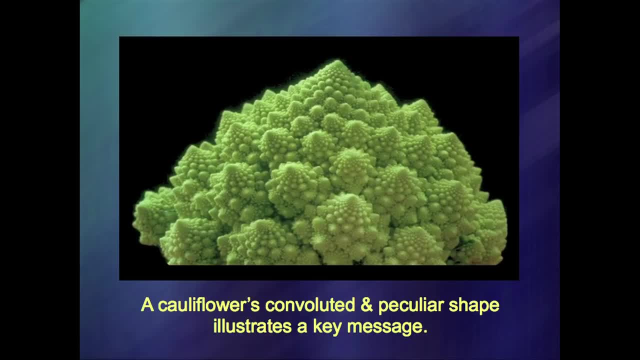 in a certain sense- And now this is very real- It's a cauliflower. Now why do I show a cauliflower, A very ordinary, ordinary cauliflower, A very ordinary and ancient vegetable? Because, ordinary and ancient as it may be, it's very. 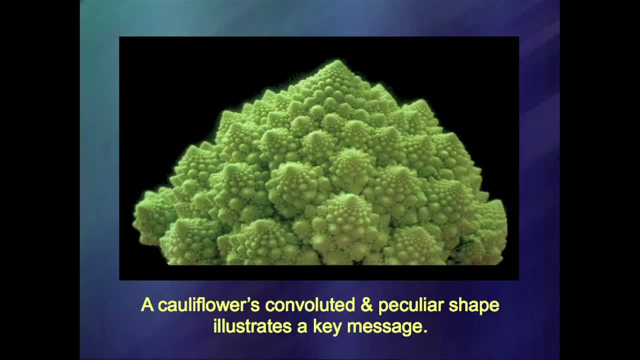 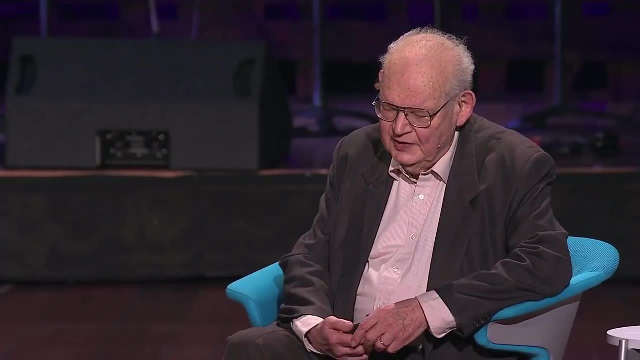 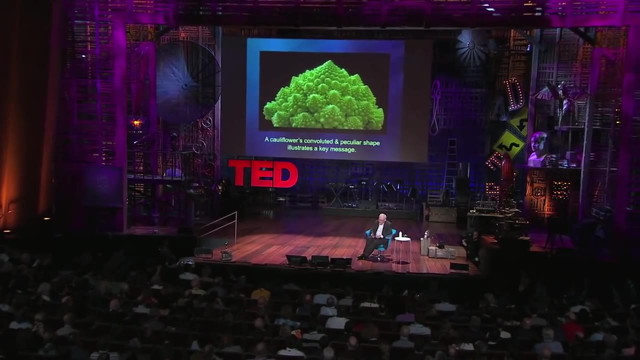 complicated and it's very simple both at the same time. If you try to weigh it, of course it's very easy to weigh it, And when you eat it, then the weight matters. But suppose you try to measure its surface. Well, it's very interesting If you cut with a sharp. 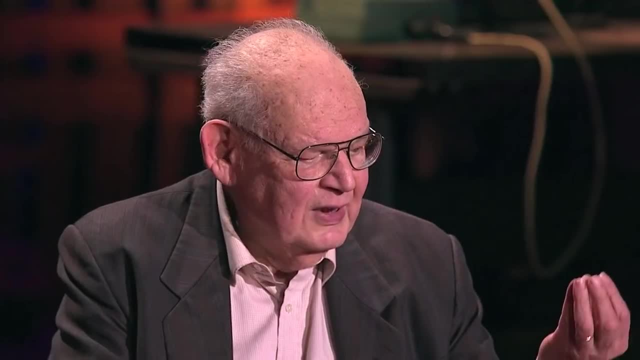 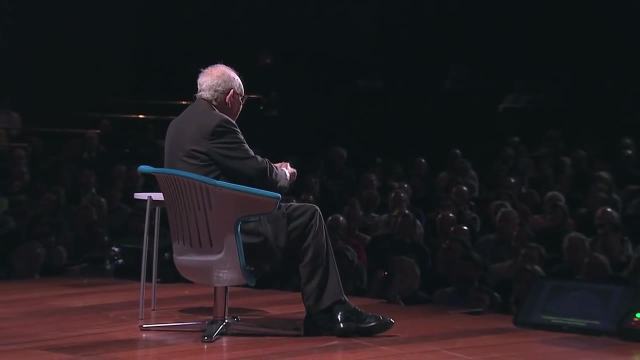 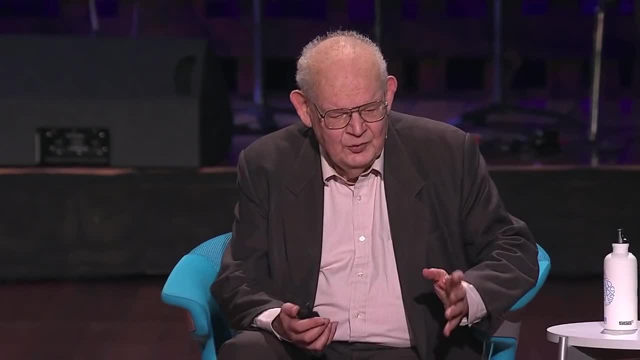 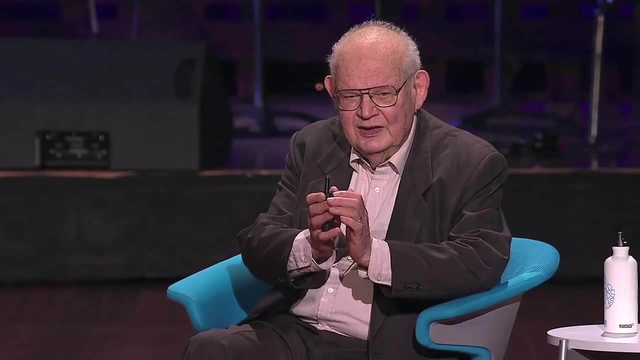 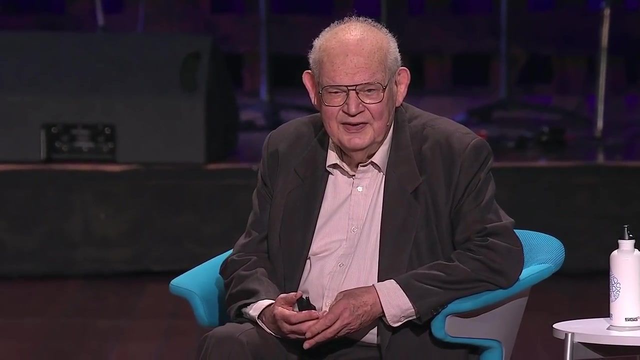 small cauliflowers. So the experience of humanity has always been that there are some shapes which have this peculiar property that each part is like the whole but smaller. Now, what did humanity do with that? Very, very little So. 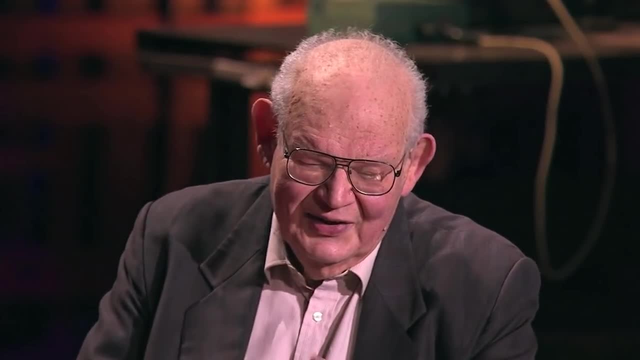 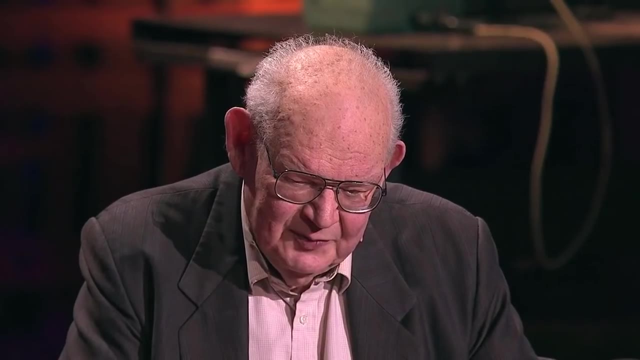 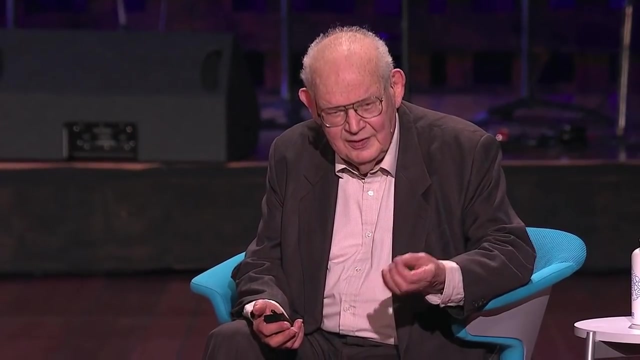 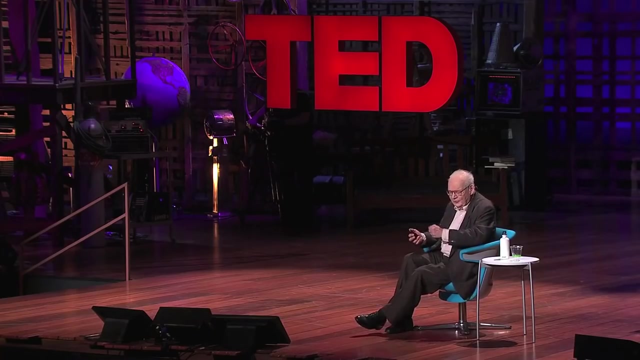 So, So, So What I did actually is to study this problem and found something quite surprising: that one can measure roughness by a number. a number 2.3,, 1.2, and sometimes much more. One day, a friend of mine to bug me, brought a picture and said: what is the roughness? 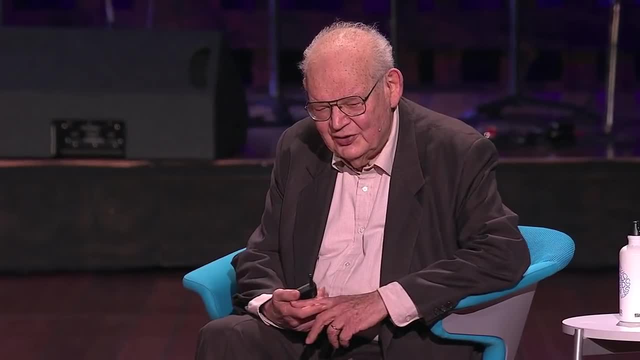 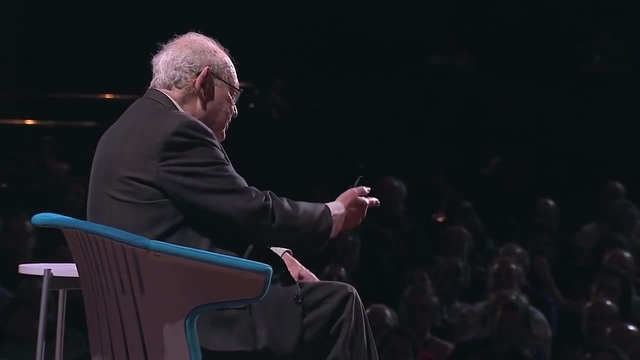 of this curve, I said: well, just short of 1.3.. Just short of 1.5., It was 1.48.. Now it didn't take any time- I've been looking at these things for so long- that these numbers 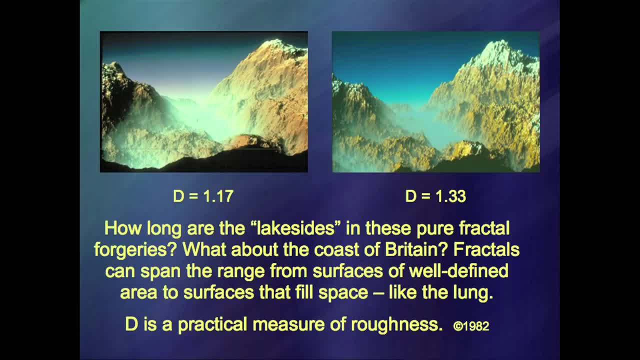 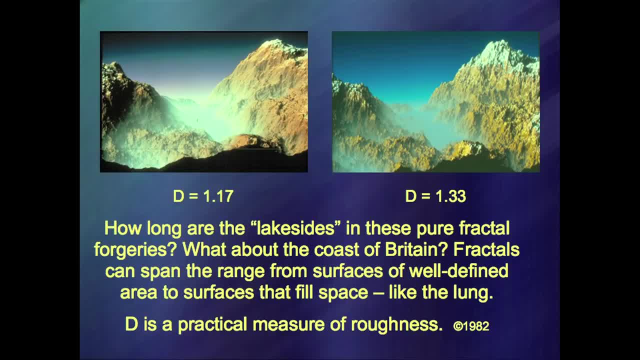 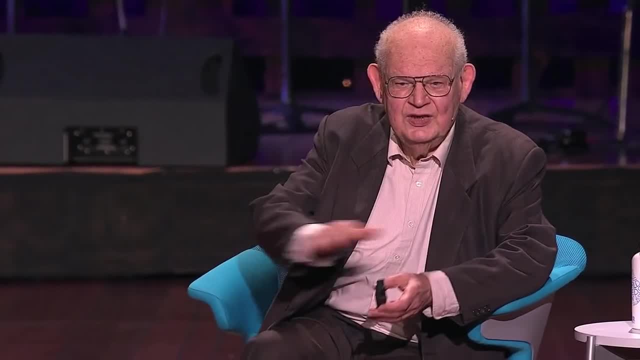 To the right I took the roughness copied from many landscapes. To the right I took the higher roughness. So the eye after a while can distinguish these two very well. Humanity had to learn about measuring roughness. This is very rough and this is sort of smooth. 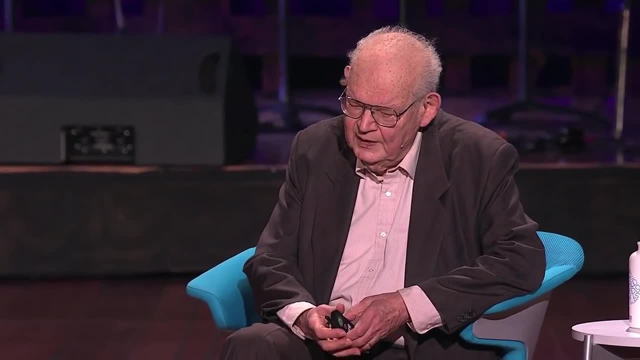 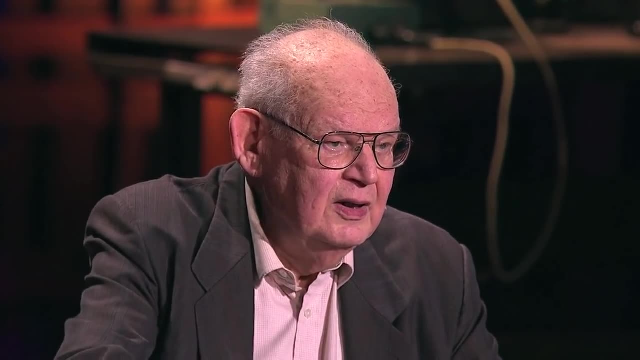 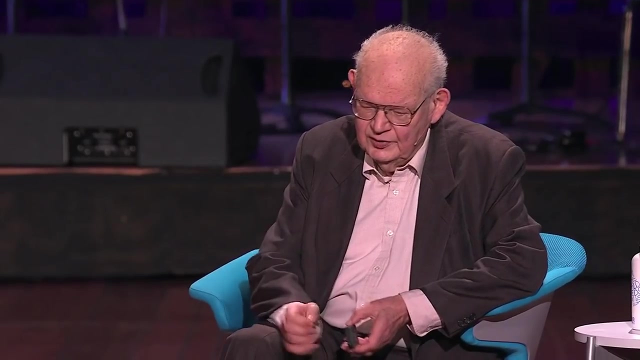 and this is perfectly smooth. Very few things are very smooth. So if you try to ask questions, how was surface a cauliflower? Well, you measure, and measure, and measure. Each time you look closer it gets bigger, down to very, very small distances. 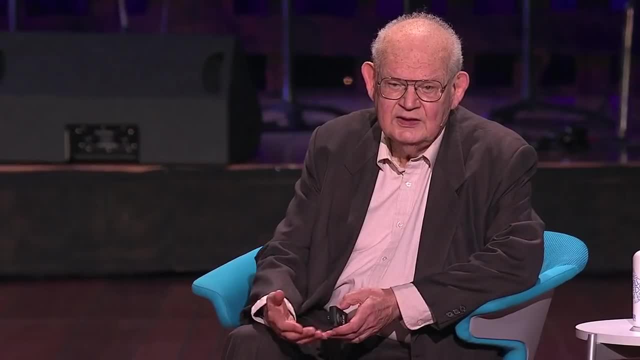 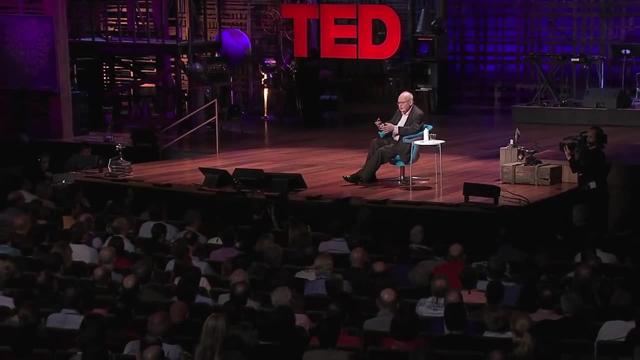 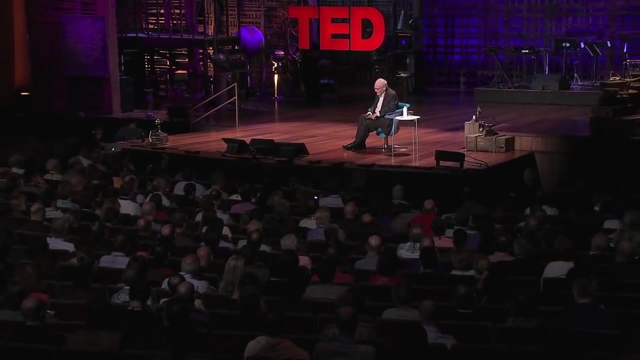 What's the length or coastline of these lakes? The closer you measure, the longer it is. The concept of length or coastline, which seems to be so natural because it's given in many places, is in fact complete fallacy. There's no such thing. You must do it differently. 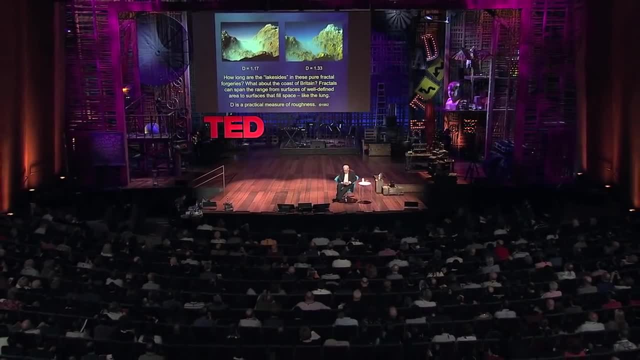 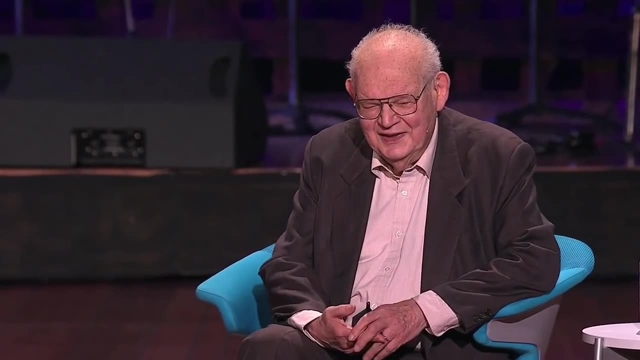 What good is that to know these things? Well, surprisingly enough, it's good in many ways. To begin with, the artificial landscapes which I invented, sort of, are used in the cinema all the time, When you see mountains in distance. they may be mountains, but they. 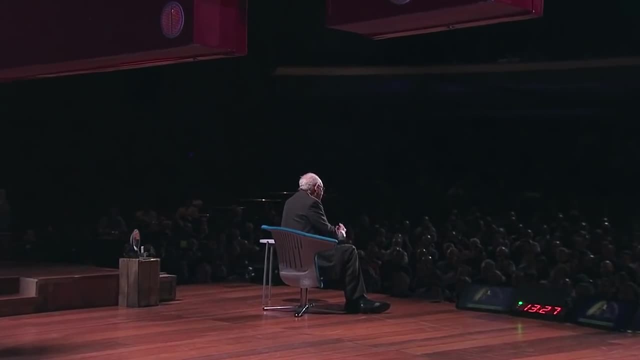 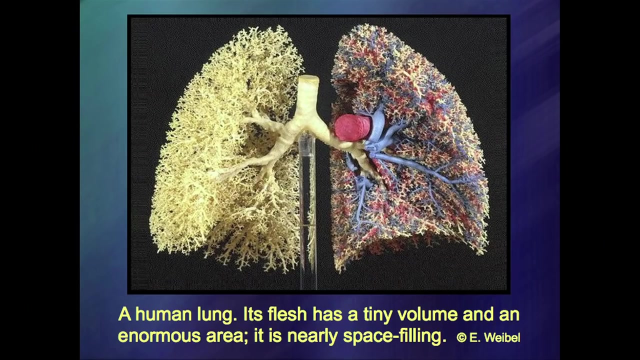 may be just a formula just cranked on. Now it's very easy to do. It used to be very time-consuming, but now it's nothing Now. look at that. That's a real lung. Now, a lung is something very 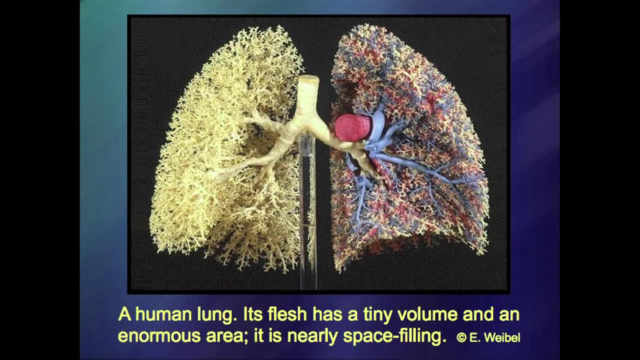 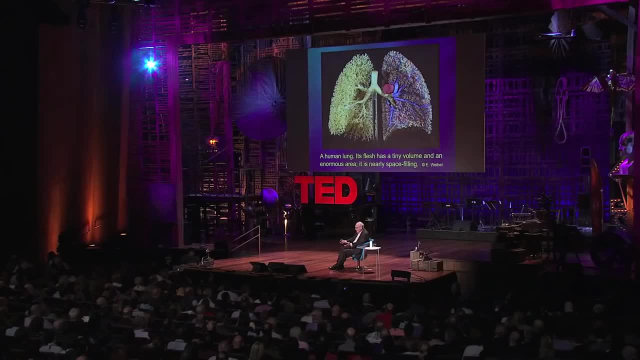 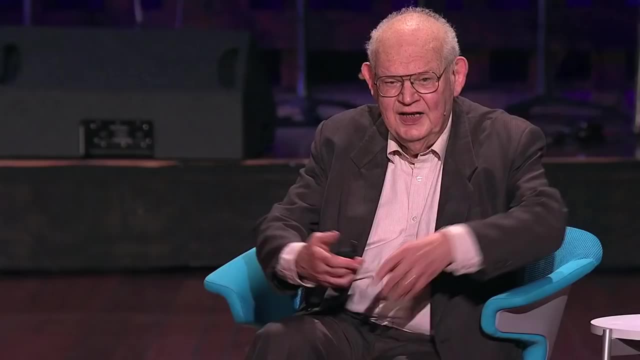 strange. If you take this thing, you know very well it weighs very little. The volume of a lung is very small. But what about the area of the lung? Anatomists were arguing very much about that. Some say that normal males' lung has an area inside of a basketball and the others say 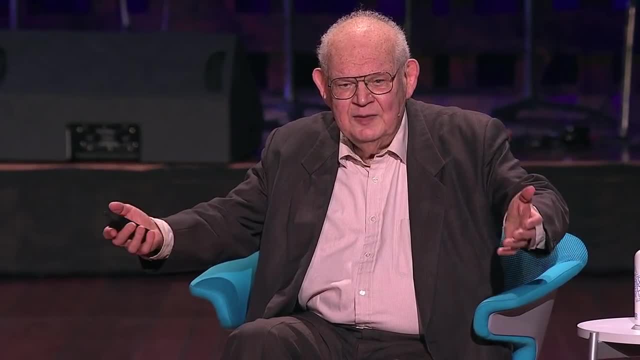 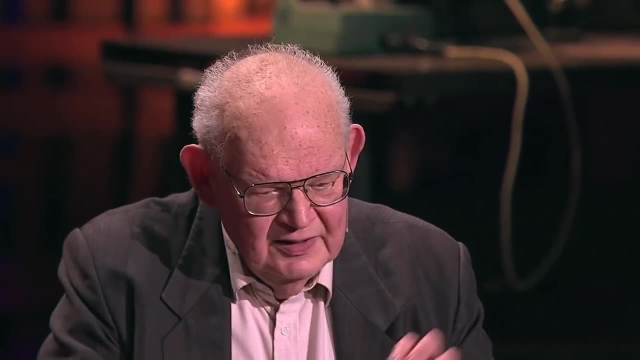 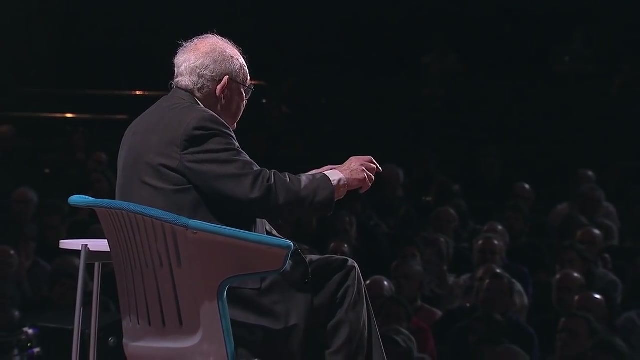 no five-up basketballs. Enormous disagreements. Why so? Because, in fact, the area of the lung is something very ill-defined. The bronchi branch, branch, branch, and they branch, not because – and they stop branching not because of any matter of principle, but because of. 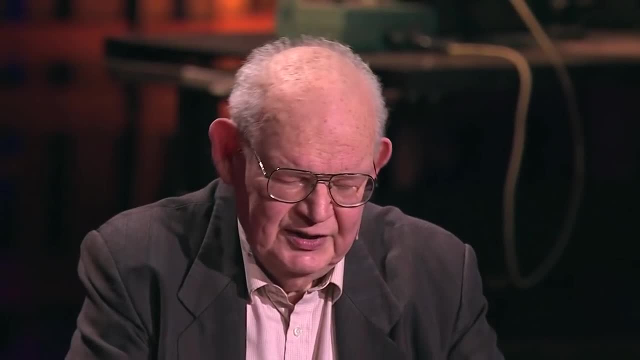 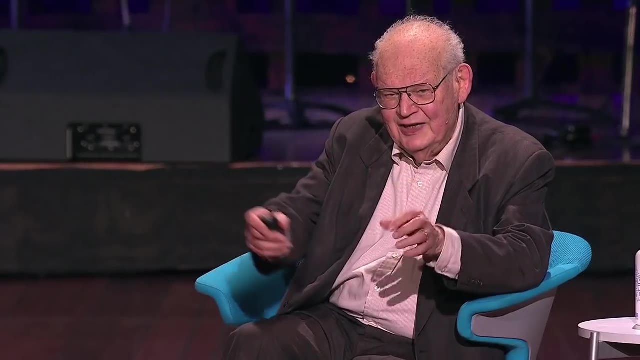 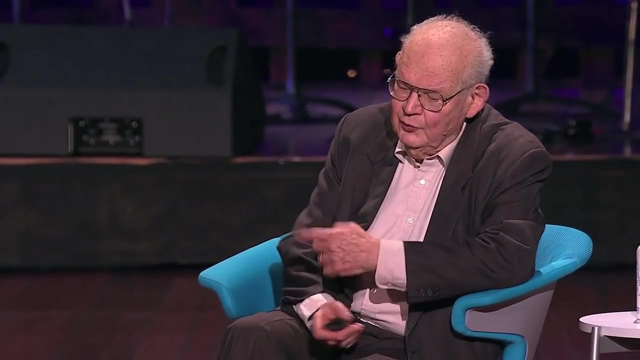 physical consideration, the mucous which is in the lung. So what happens is that a whale would have a much bigger lung, but it branches and branches down to distances about the same for a whale, for a man and for a little rodent. So now 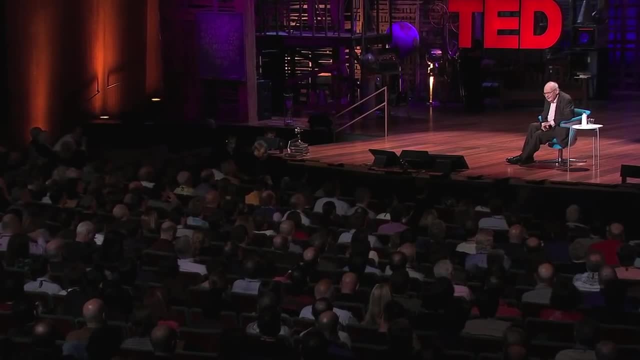 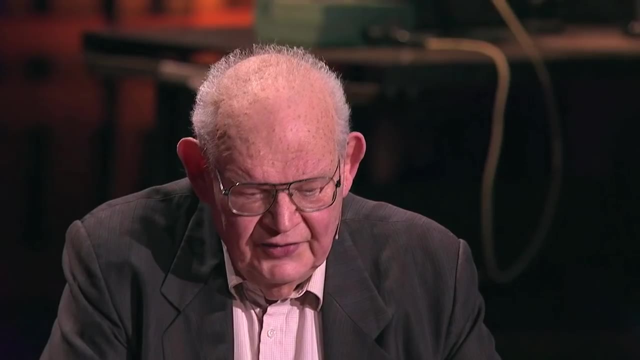 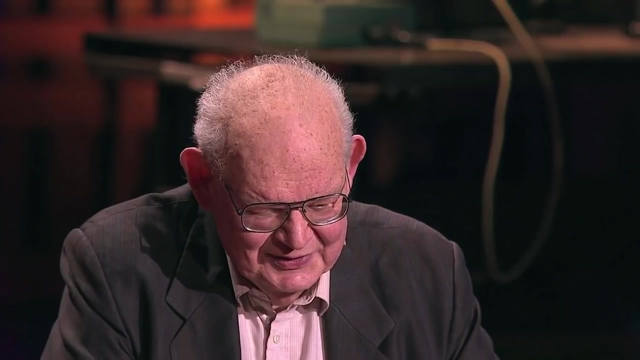 what good is it to have that? Well, surprisingly enough, amazingly enough, the anatomists had a very poor idea of the structure of the lung until very recently, And I think that my mathematics, surprisingly enough, has been of great help to the surgeons studying lung illnesses and 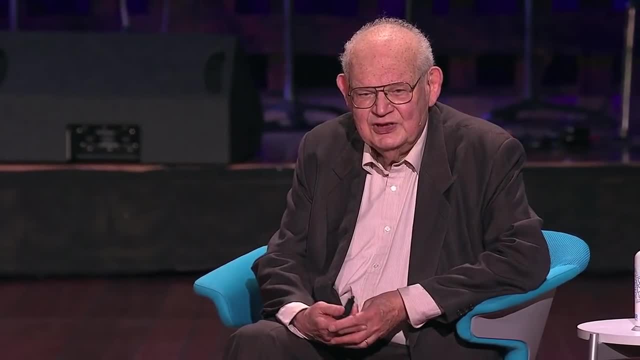 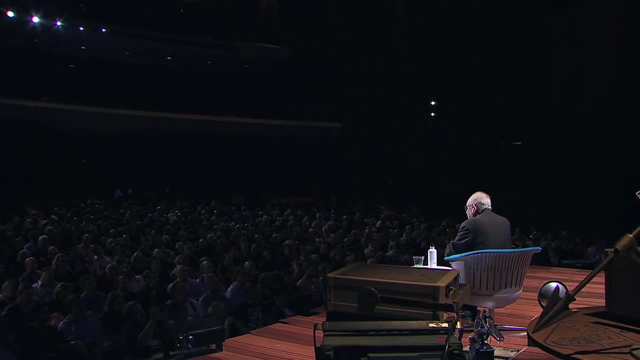 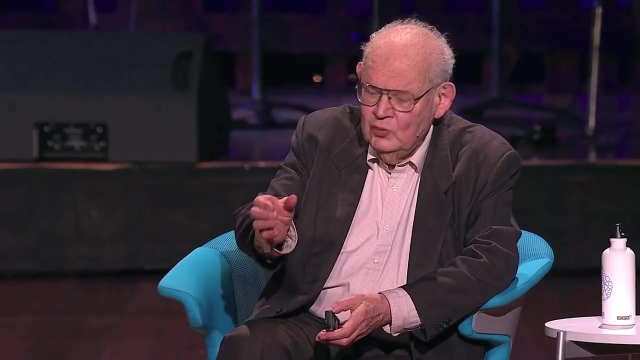 also kidney illnesses, all these branching systems which were – for which there was no geometry. So I found myself, in other words, constructing a geometry, a geometry of things which had no geometry, And the surprising aspect of it is that, very often, the rules of this geometry are extremely short. You have formulas that 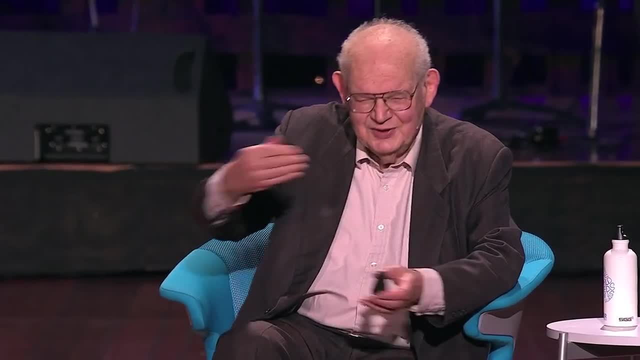 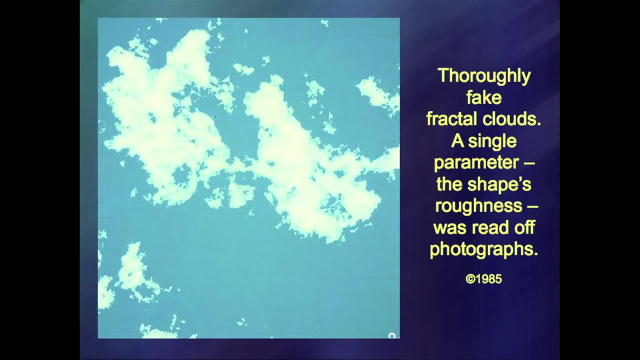 long And you crank it several times, sometimes repeatedly, again, again, again, the same repetition, And at the end you get things like that: This cloud is completely 100 percent artificial. Well, 99.9.. And the only part which is natural is a number: the roughness. 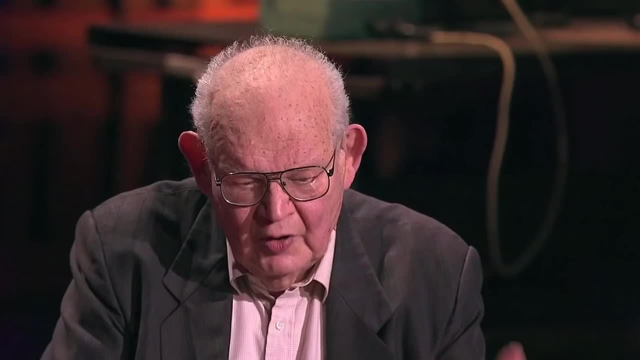 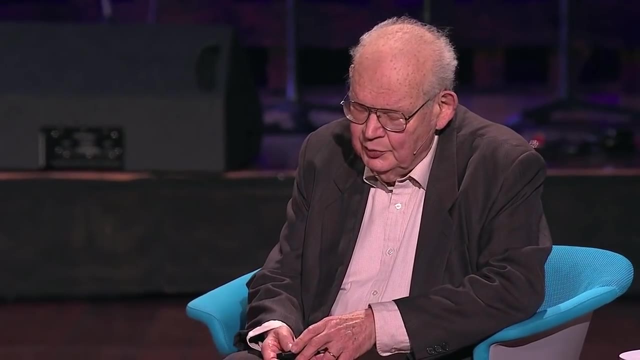 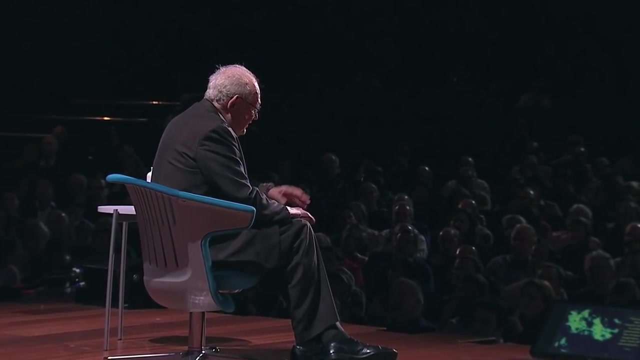 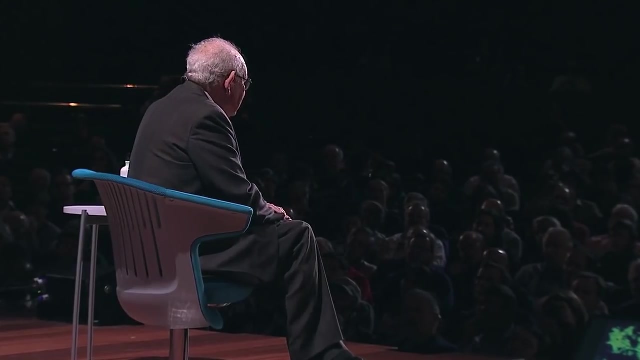 of the cloud which is taken from nature. Something so complicated, a cloud, so unstable, so varying, should have a simple rule behind it. Now, this simple rule is not an explanation of clouds, And the theory of clouds had to take account of it. I don't know how much I have advanced. This picture is rather old. 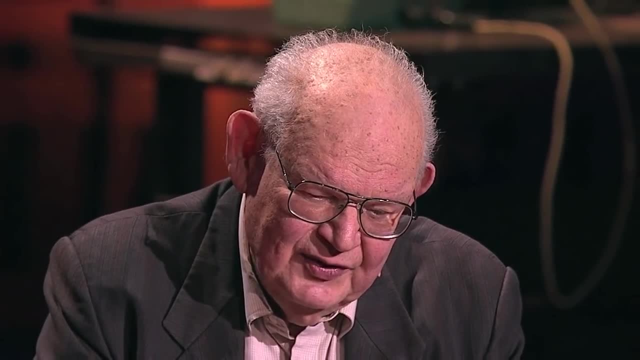 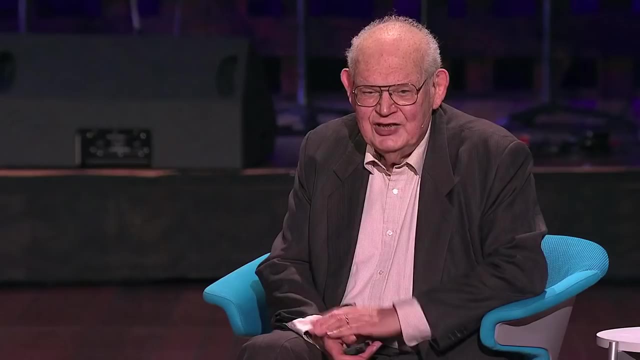 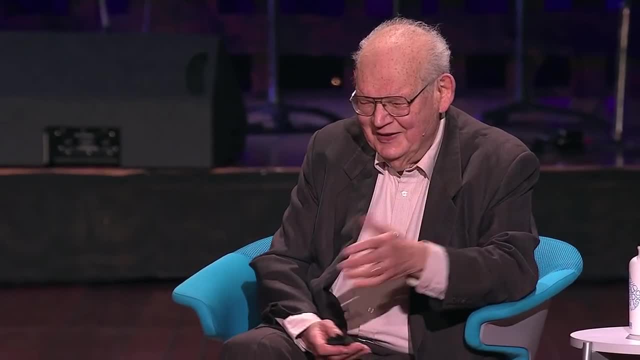 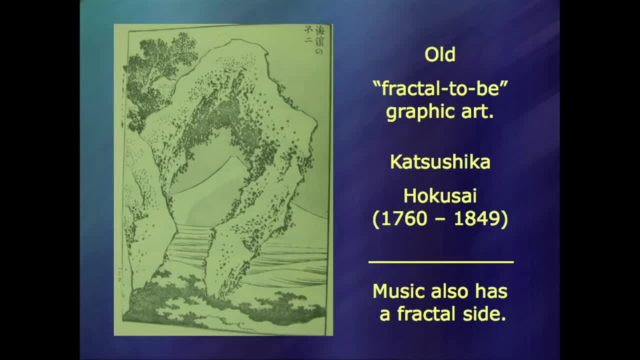 number of times, the number of times, the number of times, the number of day: DAY. So the answer S: Okay. the real thing is this: comment that Okay, Oh my, I didn't. Oh my God, Oh my God. 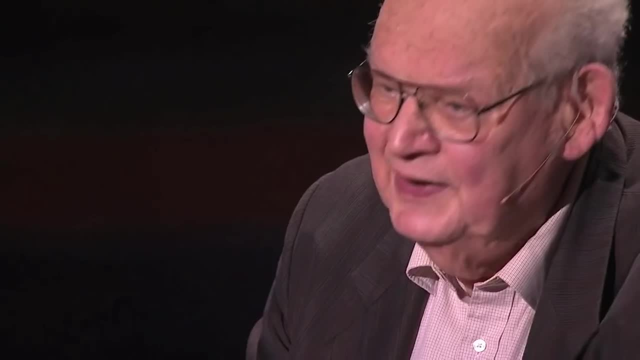 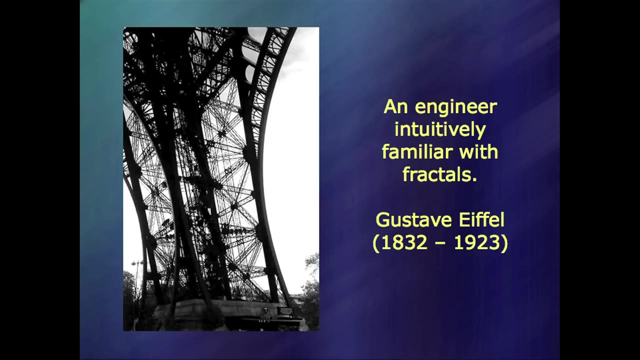 Down to the bottom. The problem- and look what I've said- is that the산 t, not t, t, tn. It's not, That's not. The question is not. Yes, maybe h1.. So in this way, the 활동 was caused by two clickers. 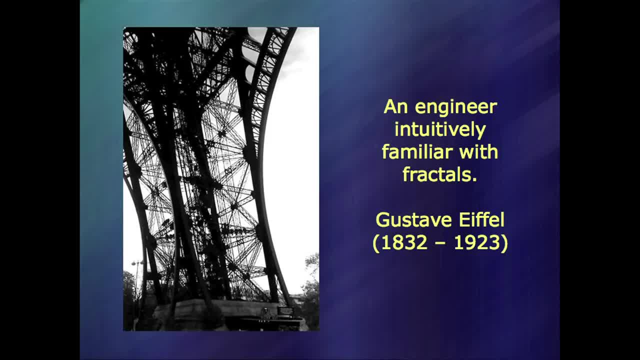 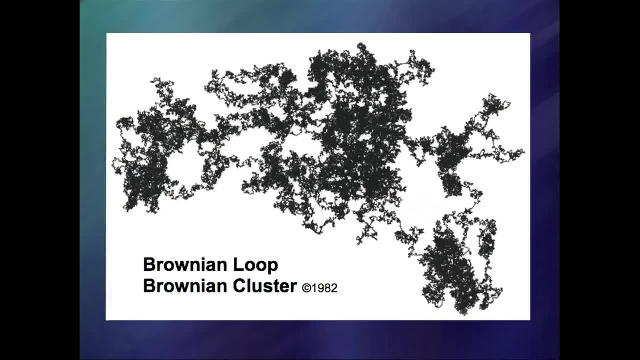 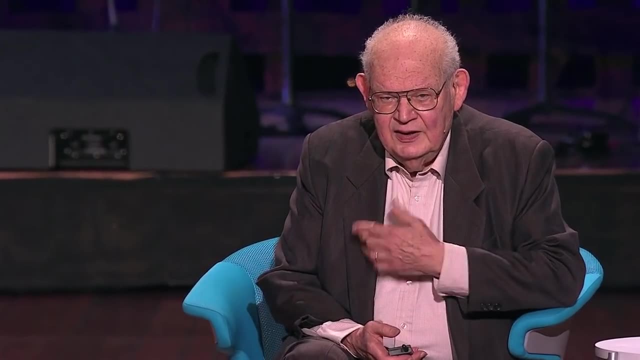 h1?? Yes, tahms, Yes, indeed, he was4. he understood This is a mess, mess, mess. Brian Loop. One day I decided halfway through my career I was helped by so many things in my work- I decided to test myself Could. 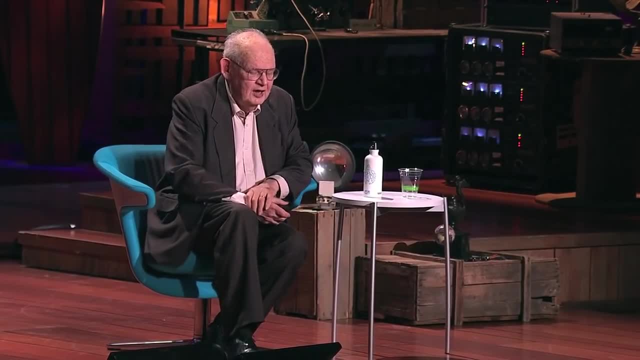 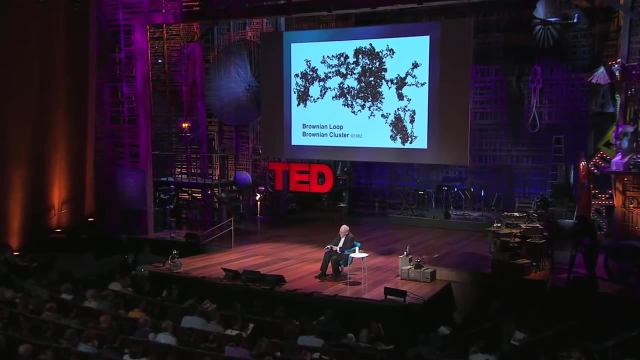 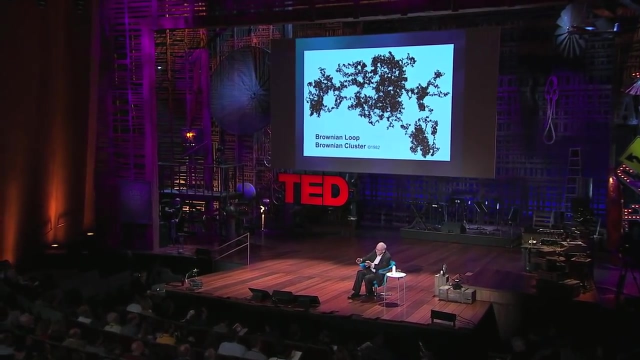 I just look at something which everybody had been looking at for a long time and find something geometrically new. Well, so I looked at this thing called Brian. Motion just goes around, I made it, I played with it for a while, then I made it return to the origin. Then I was. 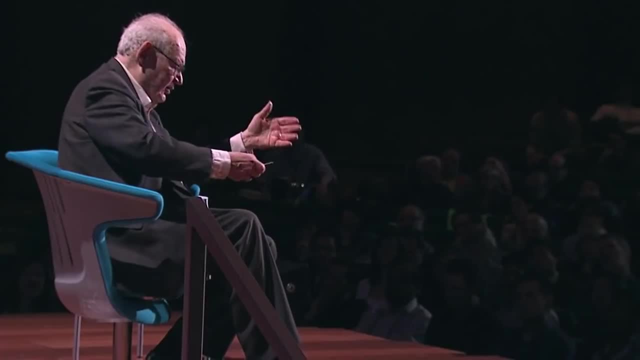 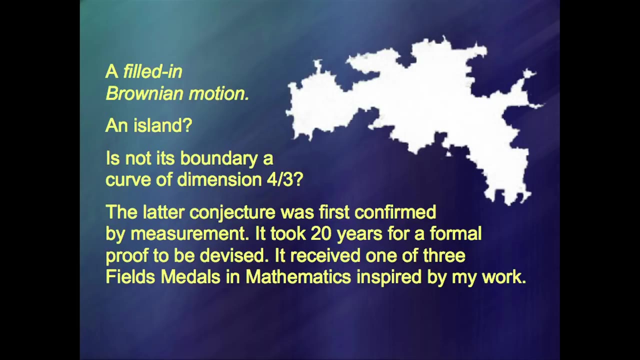 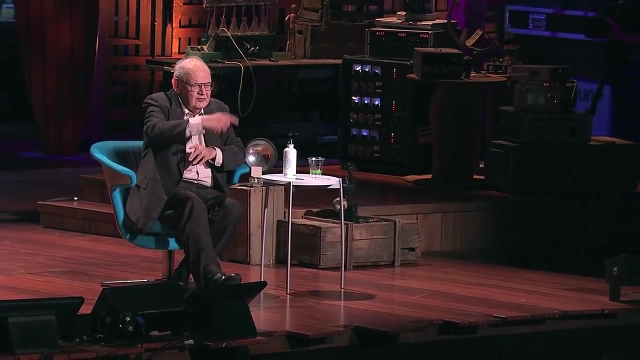 telling my assistant: I don't see anything, Can you paint it? So he painted it, which means that he put inside everything inside. When this thing came out, I said stop, stop, stop. I see it in Ireland. And then, amazing. so Brian Motion, which happens to have roughness. 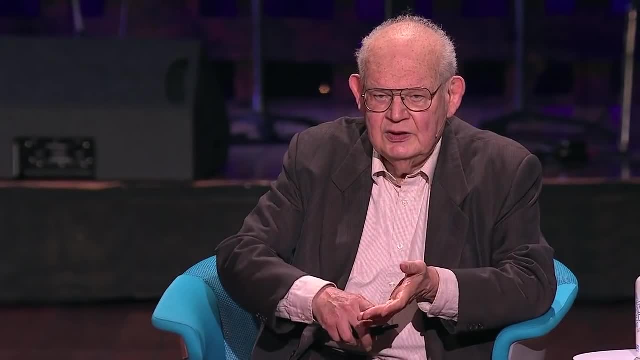 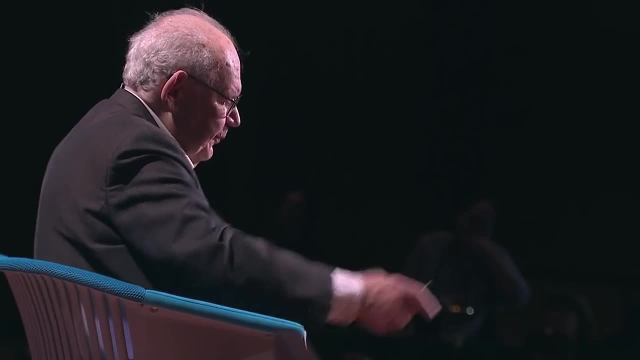 of number two goes around. I measured it 1.33, again, again, again, again, again, and again, again, again and again, and again and again. I had long measurements. big Brian Motion, 1.33.. Mathematical problem. how to prove it? It took my friends 20 years Three. 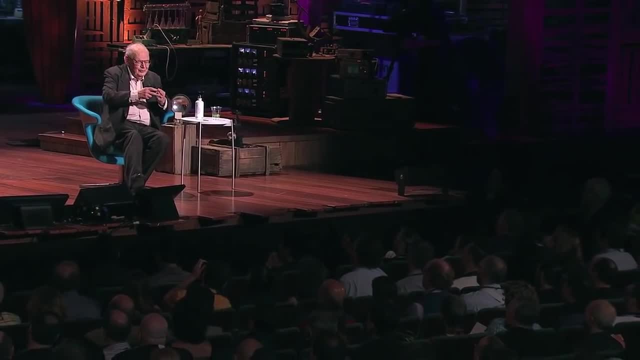 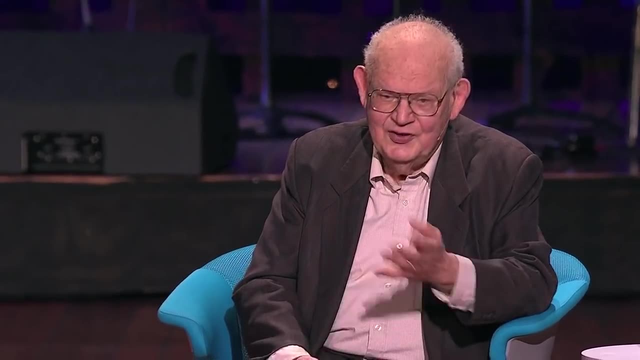 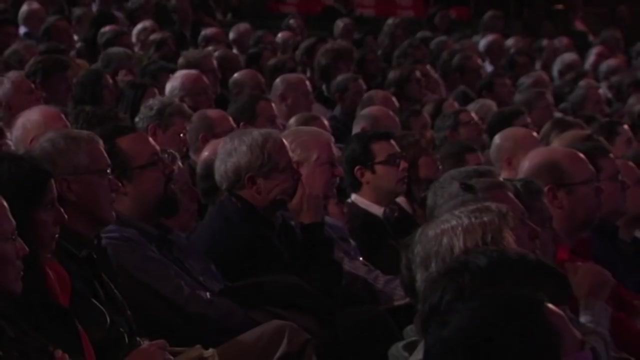 of them were having incomplete proofs. they got together and together they had the proof. So they got a big medal in mathematics, one of the three medals that people received for proving things which I've seen without being able to prove them. Now everybody had asked. 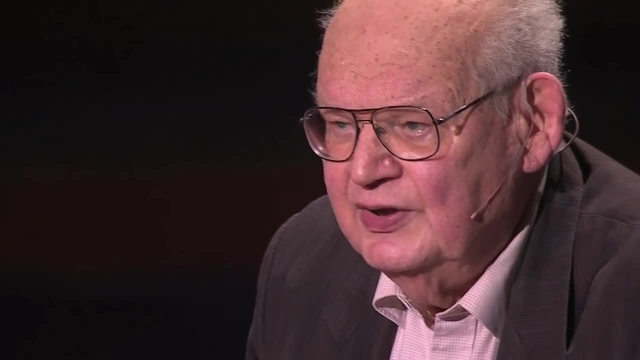 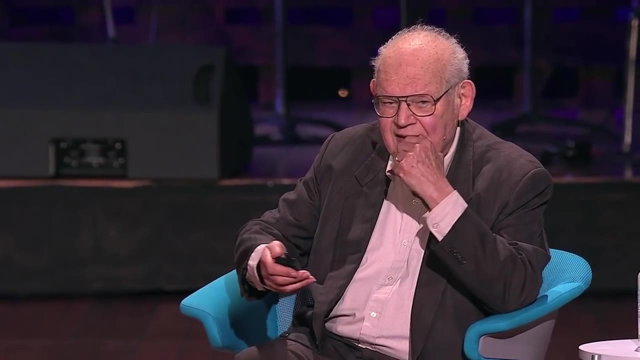 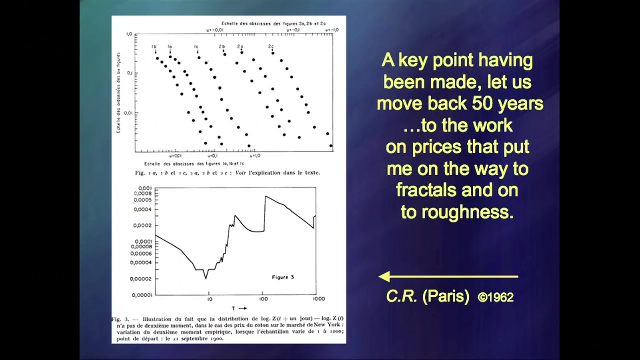 point to another. how did it all start? What got you in that strange business? What got you to be, at the same time, a mechanical engineer, a geographer and a mathematician, and so on, and a physicist? Well, actually I started, oddly enough, studying stock market prices. 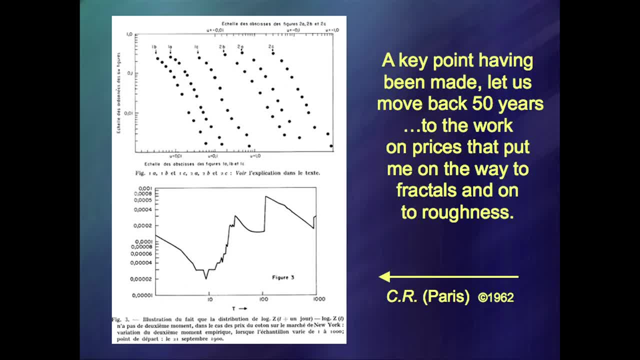 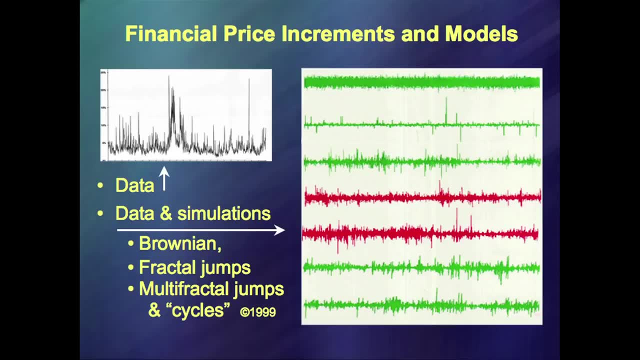 And so here I had this, developed this theory and I wrote books about it. Financial prices increments. To the left, you see data over a long period. To the right, on top, you see a theory which is very, very fashionable Because it's very easy. you can write many. 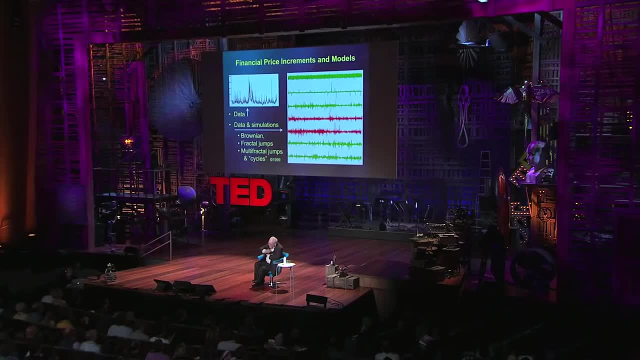 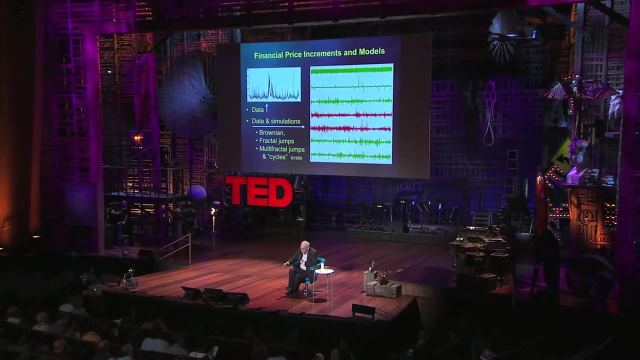 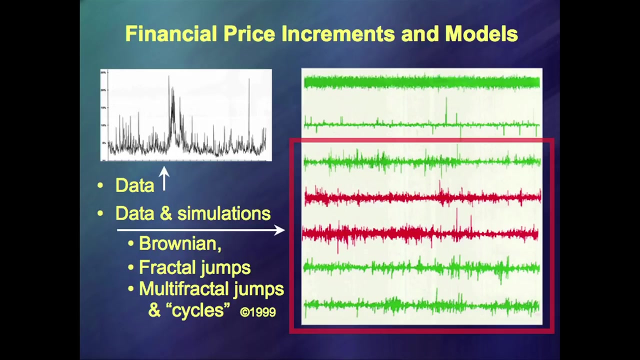 books very fast about it, So thousands of books on that. Now compare that with the real price increments. And where are real price increments? Well, these other lines include some real price increments and some forgery, which I did. So the idea there was. 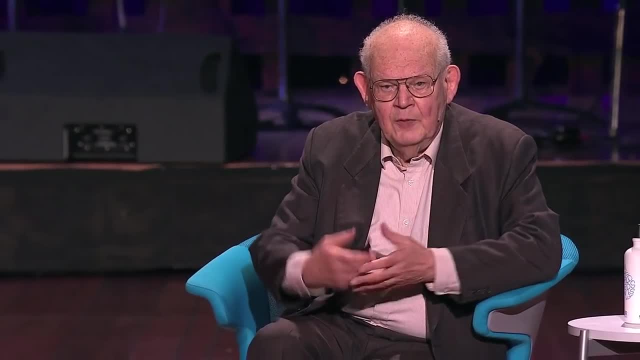 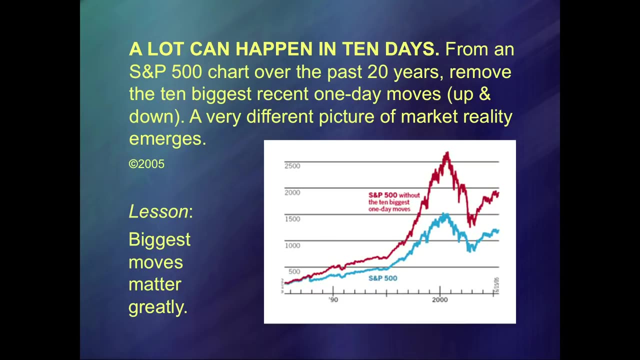 that one must be able to understand the real price increments. So I started to how to say model price variation And it went extremely well 50 years ago. For 50 years people were sort of poo-pooing because they could do it much, much, much. 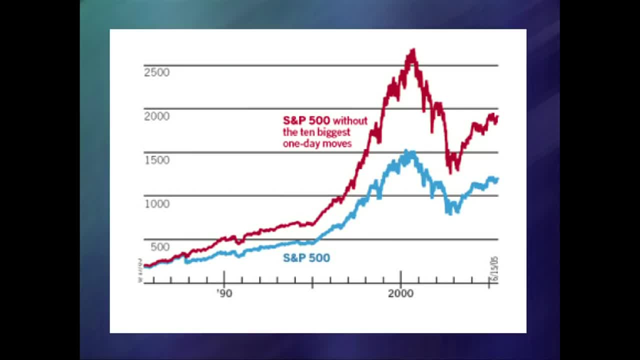 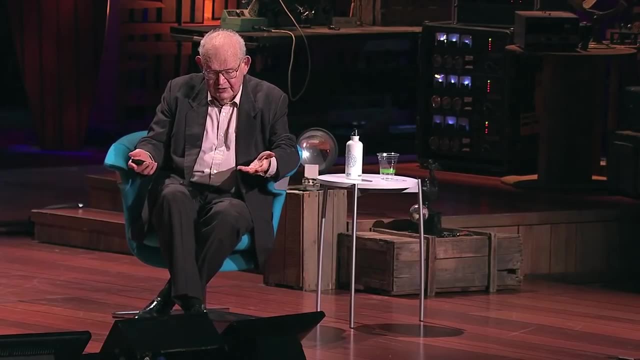 easier. But I tell you at this point- people listen to me- These two curves are averages, standard and poor. the blue one And the red one is standard and poor, from which the five biggest discontinuities are taken out. Now, discontinuities are a nuisance. 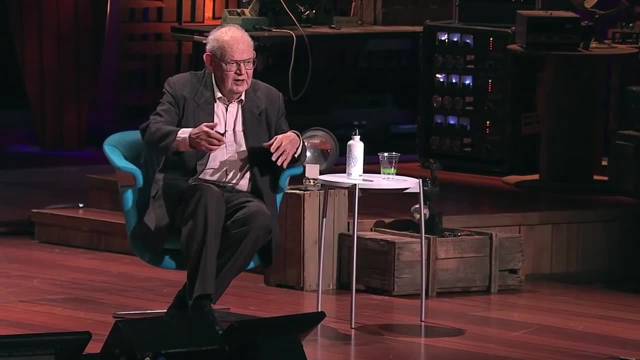 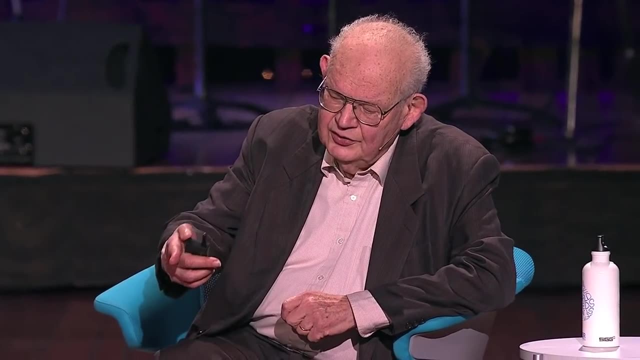 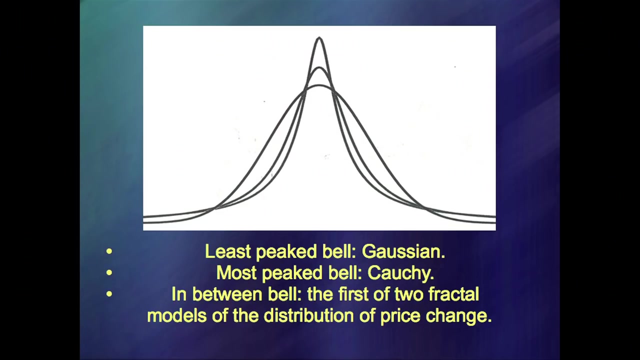 So, in all of many studies of prices, one puts them aside. Well, acts of God, and you have the little nonsense which is left. The acts of God on this picture are five. acts of God are as important as everything else. In other words, it is not acts of God which 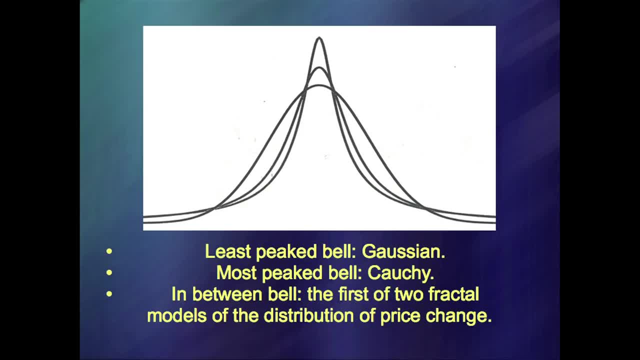 we can put aside. That is the meat. the problem, If you master these, you master price, And if you don't master this, you can master the little noise as well as you can, But it's not important. Well, here are the curves for it. 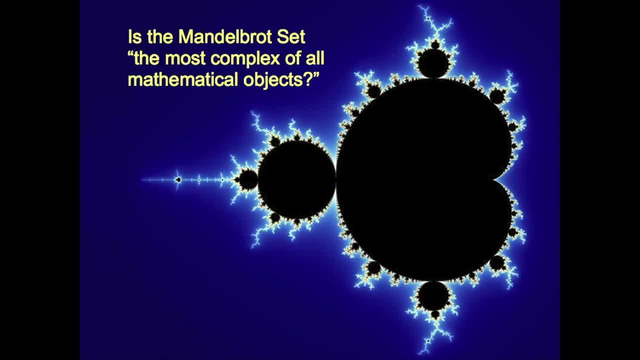 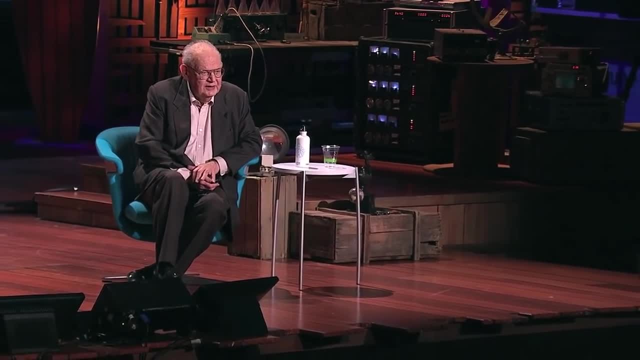 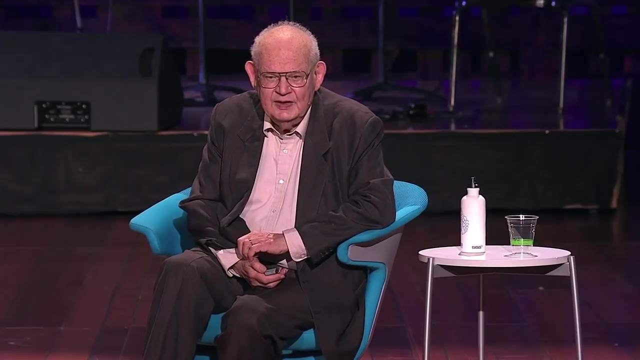 Now I get to the final thing, which is the set of which to which my name is attached. In a way, it's the story of my life. My adolescence was spent during German occupation of France And, since I thought that I may vanish within a day or the week, I had very big dreams. 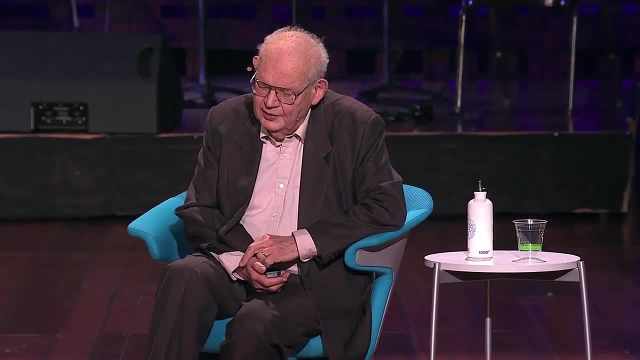 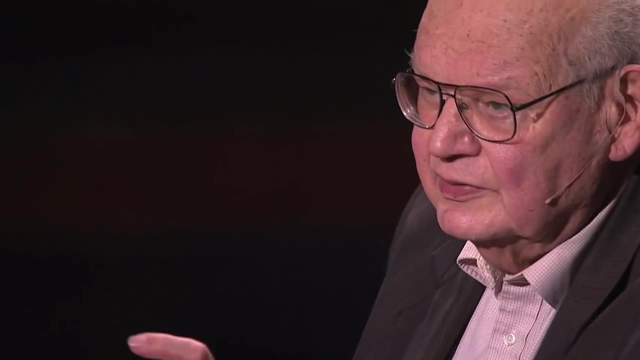 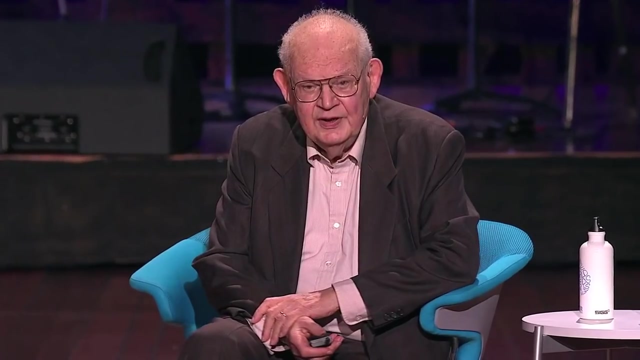 And after the war I saw an uncle again. My uncle was a very prominent mathematician And he told me: look, There is a problem which I could not solve 25 years ago and which nobody can solve. This is construction of man named Julia, and If you could find something new. 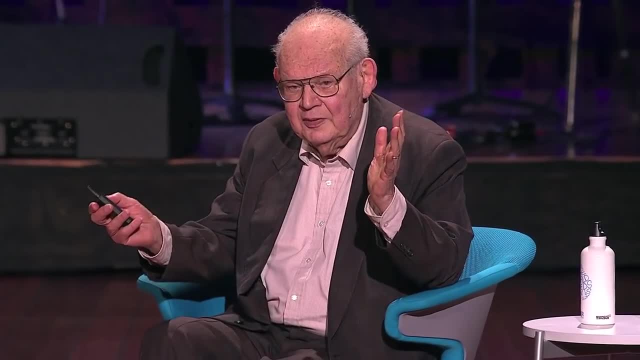 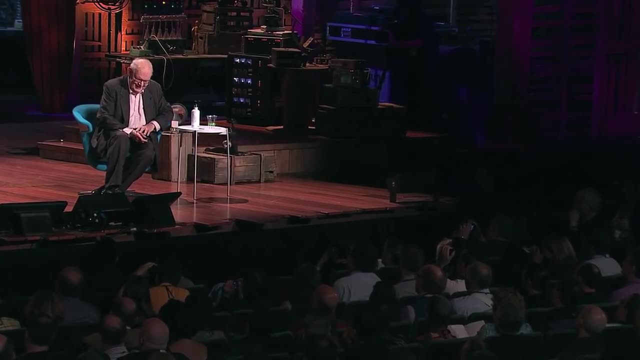 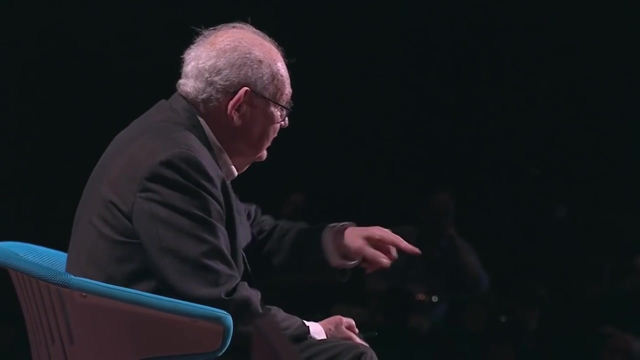 anything, you will get your career made Very simple. So I looked and, like the thousands of people I tried before, I found nothing. But then the computer came and I decided to apply computer not to new problems in mathematics but to real problems Like this wiggle. wiggle, That's a new problem, but old problems. 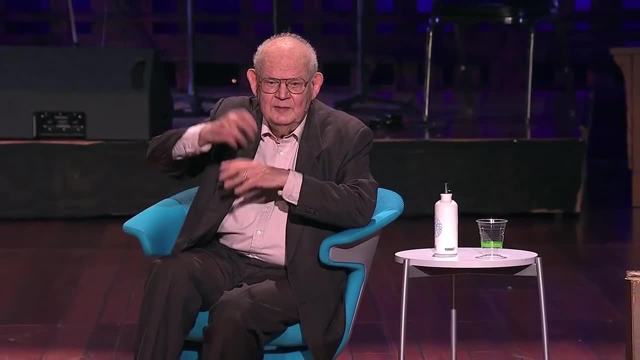 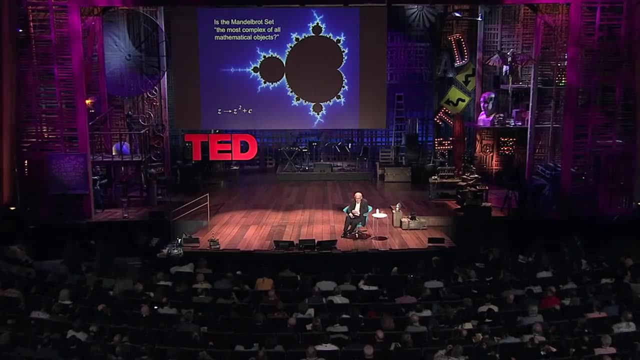 And went from what's called real numbers, which is points on a line, to imaginary, complex numbers, which are points in the plane, which is what one should do there, And this shape came out. This shape is of an extraordinary complication. The equation is written there. 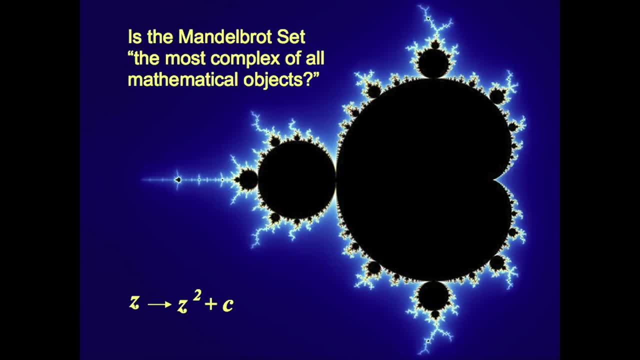 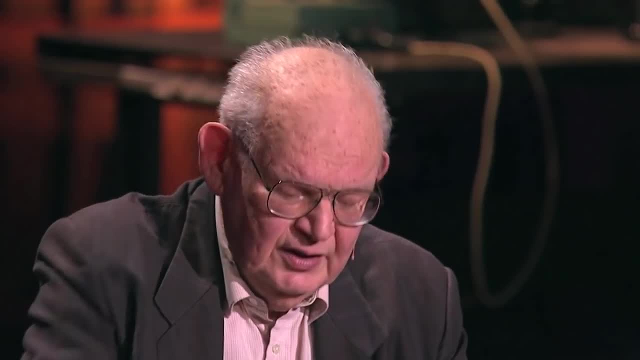 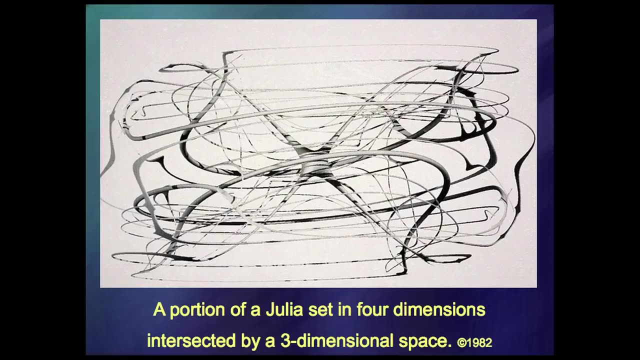 Z goes into Z squared plus C. It's so simple, is so dry, it's so uninteresting. Now you Turn the crank once, twice, twice marvels come out. I mean, this comes out. I don't want to explain these things. 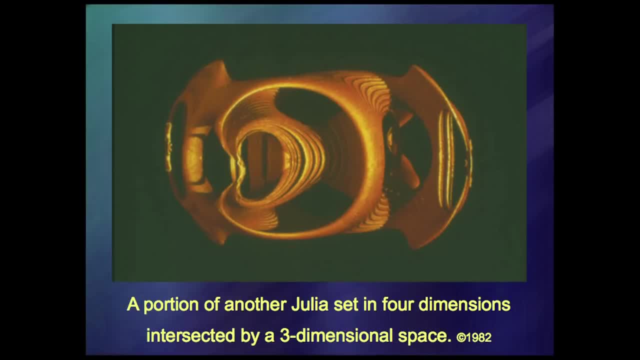 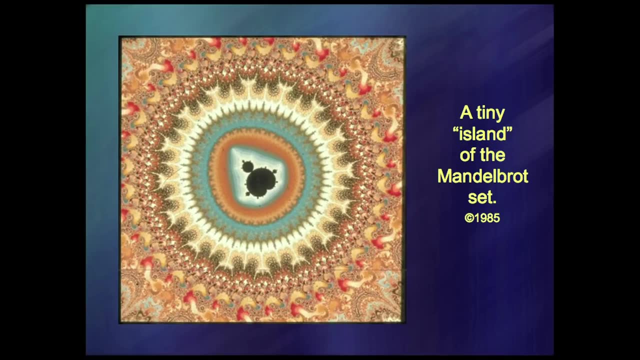 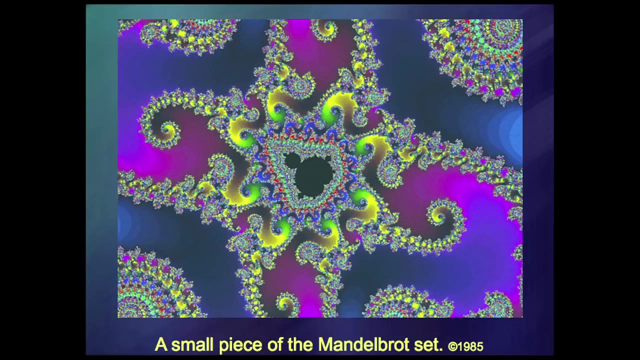 This comes out. This comes out Shapes which are of such complication, such harmony and such beauty. This comes out repeatedly, again, again, again, And that was one of my major discoveries: to find that these islands were the same as the whole big thing, more or less. 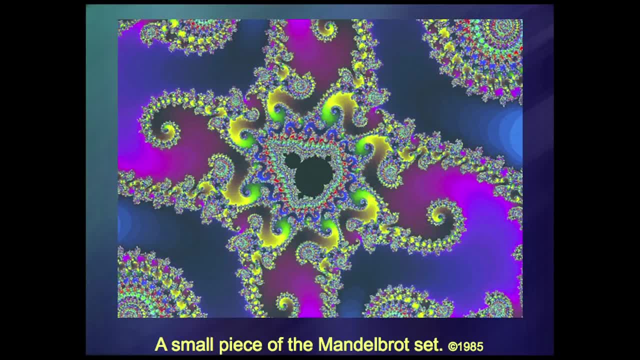 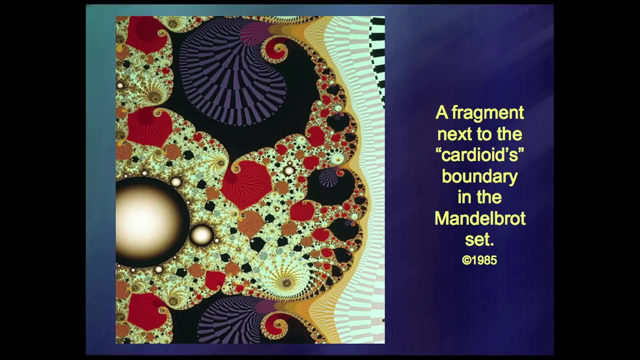 And then you get these extraordinary Baroque decoration all over the place, All that from this little formula which has whatever five symbols in it, And then this one. the color was added for two reasons. First of all, because these shapes are so complicated that one couldn't make any sense.